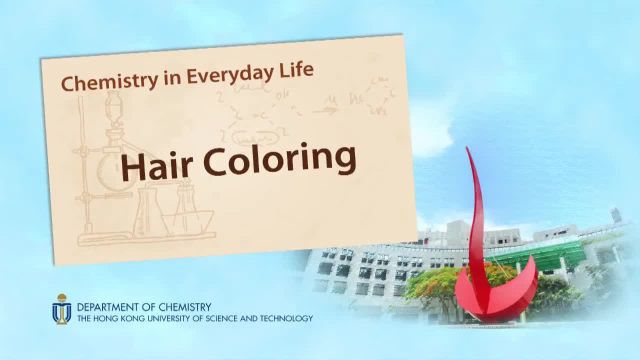 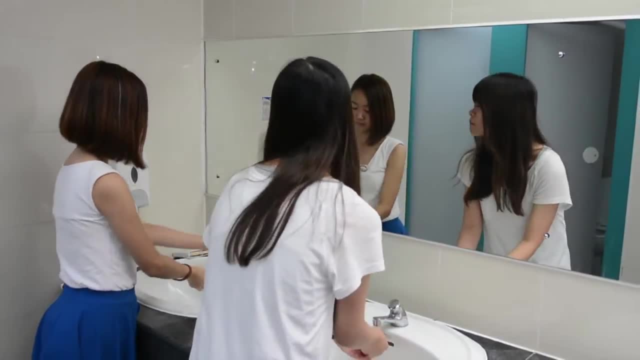 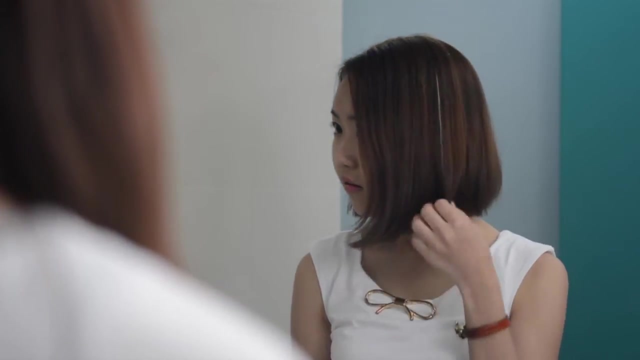 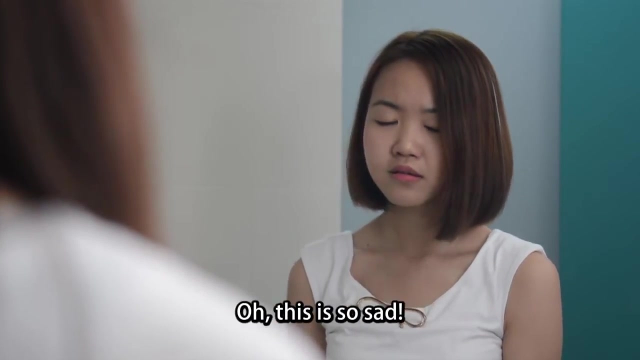 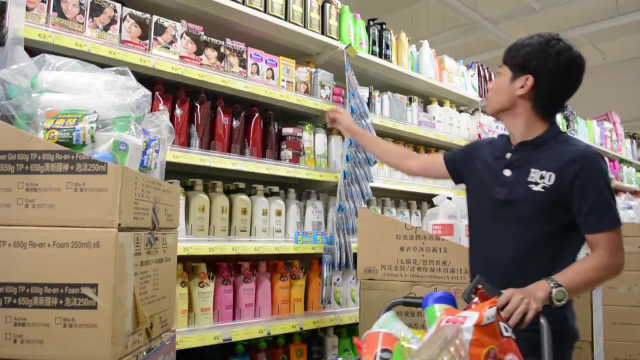 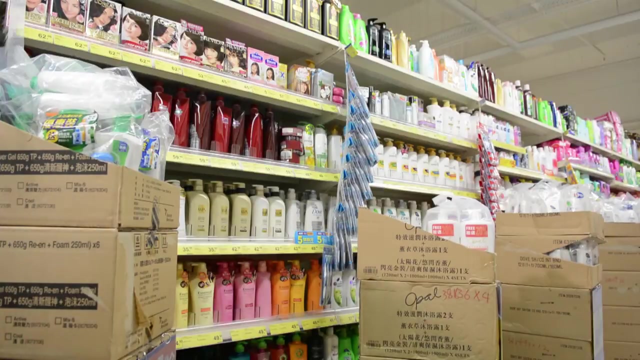 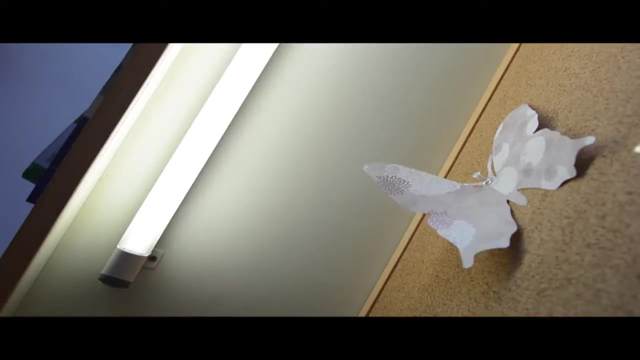 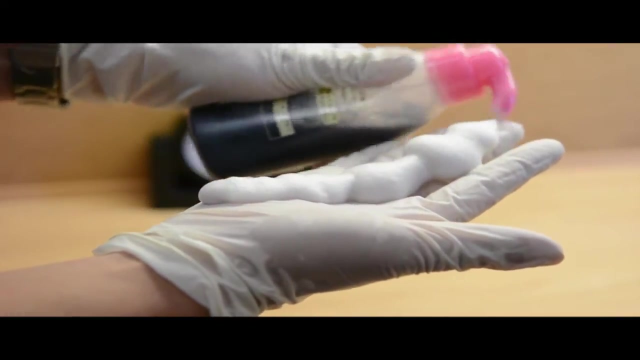 Hey, Jane is right here the new trend. You have so many of them Really. Oh my gosh. I just stayed up all night to complete two assignments. This is so sad. Clothes comb hair dye, Dr Wei, can we start? 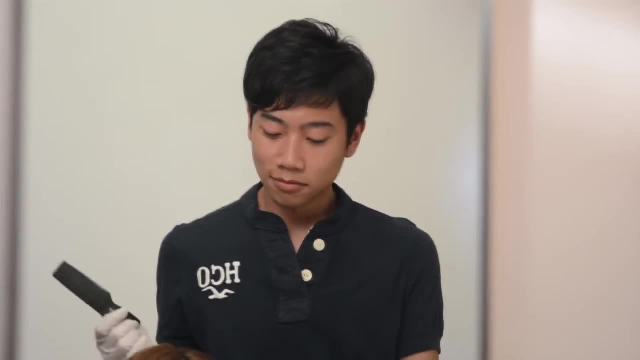 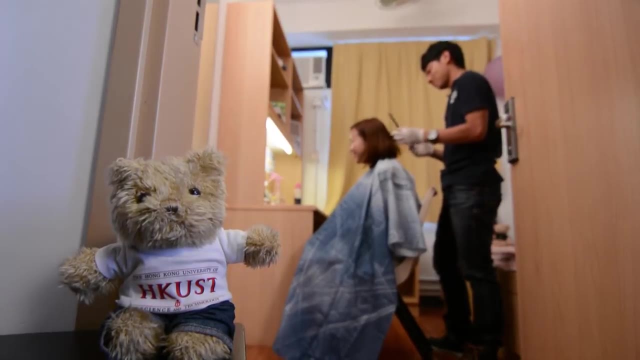 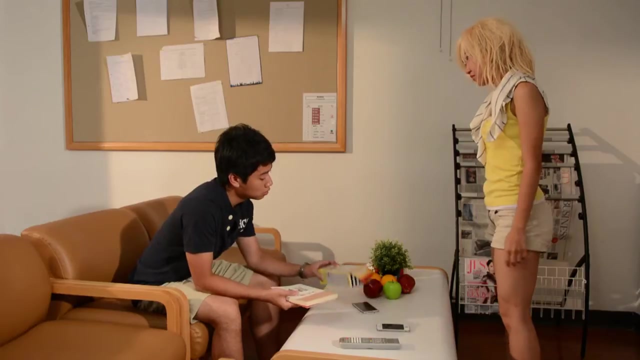 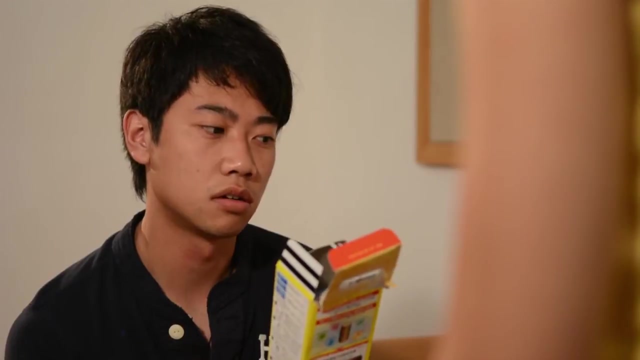 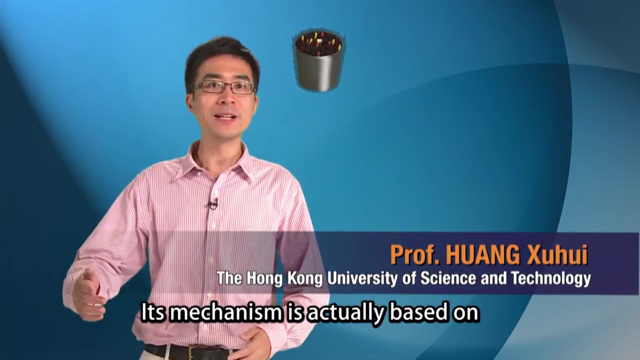 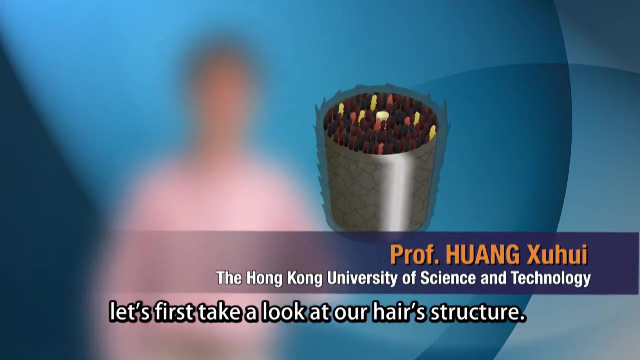 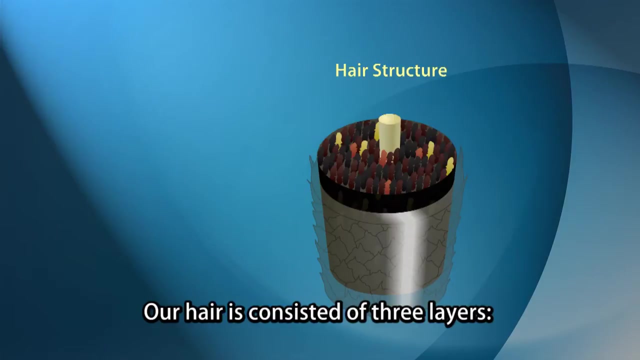 Yes. So how does hair coloring work? This mechanism is actually based on redox chemical reactions. To understand the principle of hair coloring, let's first take a look at the structure of our hair. Our hair consists of three layers: medulla, cortex and cuticle. 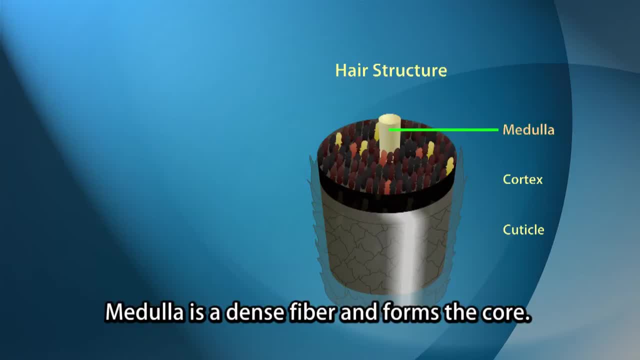 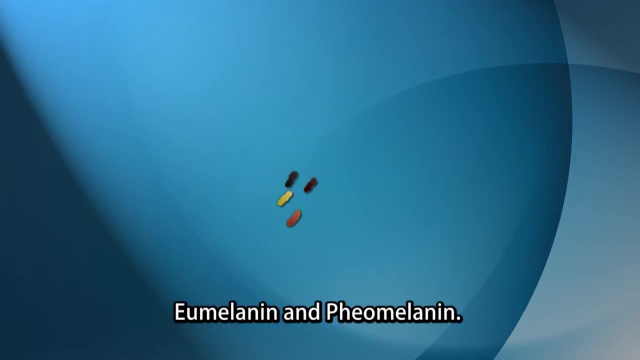 Medulla is a dense fiber and forms the core. Cortex is the middle layer and contains hair pigment that gives the color of our hair. The outer layer is thin and transparent. There exist two types of pigment in the cortex: eumelanine and pheomelanine. 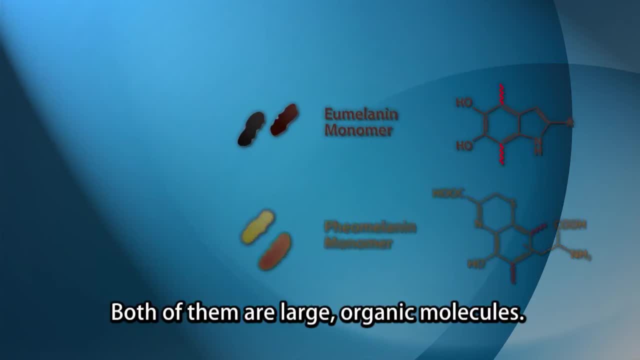 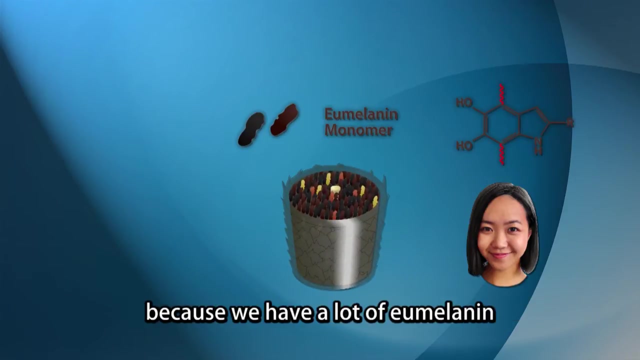 Both of them are large organic molecules. Eumelanine gives black or brown color, while pheomelanine gives yellow or red color. The ratio of these two pigments determines the color of our natural hair. For example, Asian people have black hair because we have a lot of eumelanine in our hair cortex.